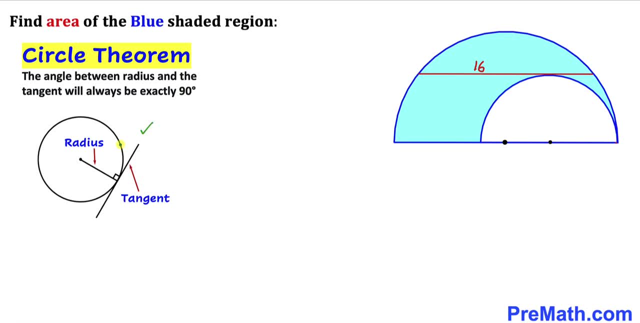 degrees, as you can see in this diagram, where this is our radius and this is our tangent line and the angle to the dotted line And the name of the circle doc argument will come from. the between them is going to be 90 degrees, so therefore the radius for this smaller. 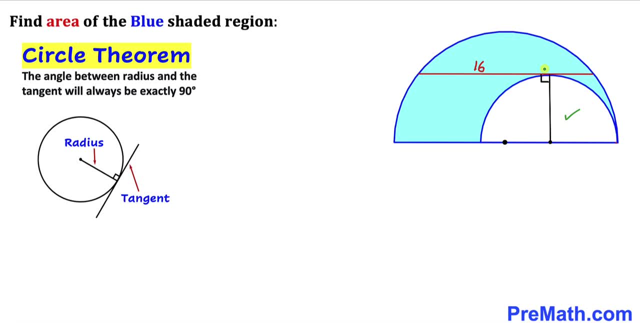 semicircle is going to be perpendicular to this cord and this angle has got to be 90 degrees and, moreover, this line is going to be perpendicular to this cord as well. since these two lines are parallel, let me call this radius for this smaller semicircle as a lowercase r, then this length is going to be: 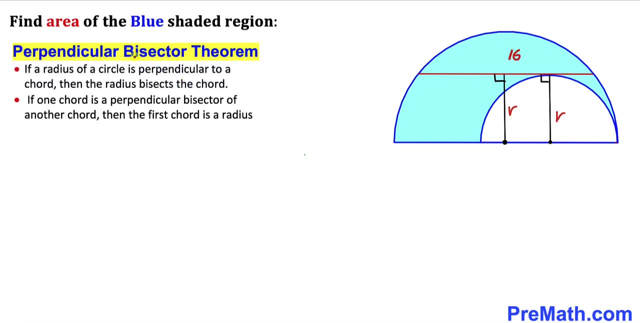 lowercase r as well. and now let's recall the perpendicular bisector theorem. if radius of a circle is perpendicular to a cord, then the radius bisects the cord, and in our case we can say that the radius of a semicircle is perpendicular to the cord, and in our case we can: 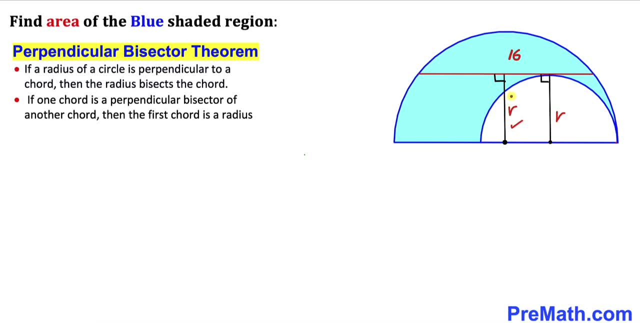 see that this line is part of the radius of this larger semicircle and this is a perpendicular to this cord. so therefore, this line is going to bisect this cord into two equal parts. if this whole length is 16 units, then this length is going to be 8, and this is going to be 8 units as well In this. 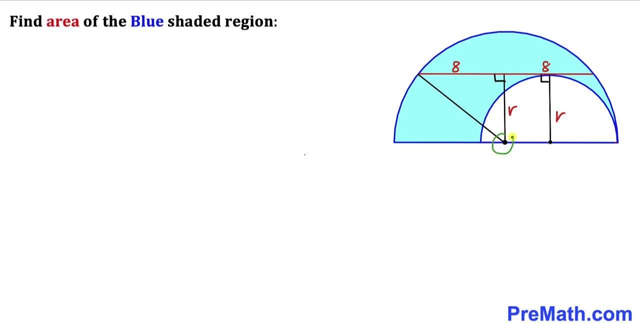 next step. I have connected these two points, this center and this point, and we can see that this is the radius of this larger semicircle. let me go ahead and represent this radius by uppercase R. and here's our much nicer looking diagram. and here's our next step. we know that the area of this blue shaded region is 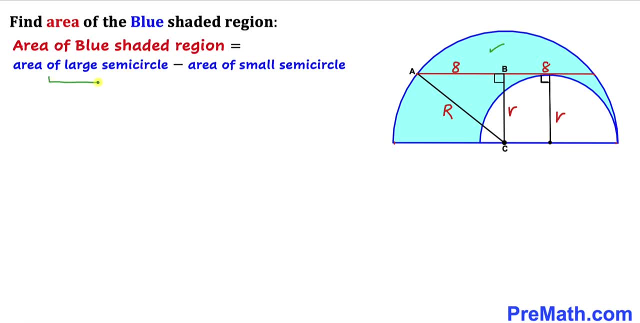 equal to the area of this larger semicircle, minus the area of this smaller semicircle. now, let's recall the area of a circle of formula area equals to PI R square. therefore, the area of semicircle is going to be PI R square divided by 2, isn't it? now let's look at the area of this larger 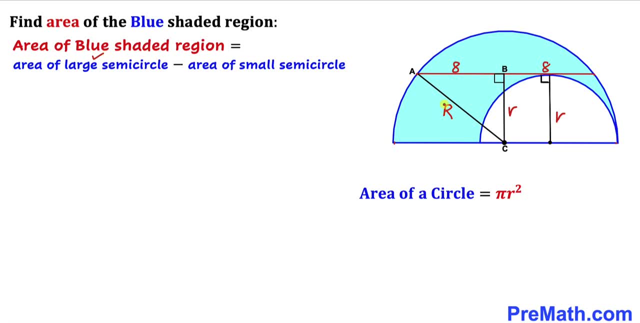 semicircle. we know that the radius is uppercase R, so the area of this larger semicircle is going to be PI R square divided by 2, and likewise the area of this smaller semicircle is going to be a PI R square divided by 2, where this 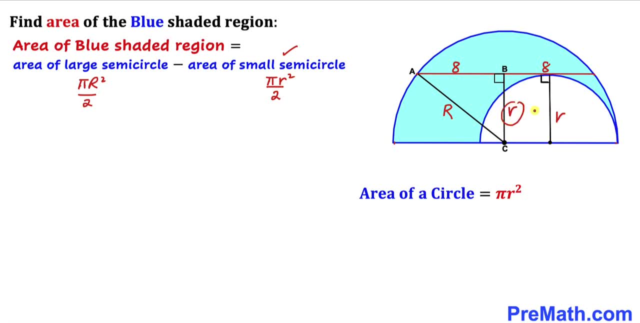 radius is lowercase R, as you can see in this next step, where this is the area of the larger semicircle minus the area of a smaller semicircle. now we can see PI divided by 2 is in common. let me go ahead and factor PI divided by 2. 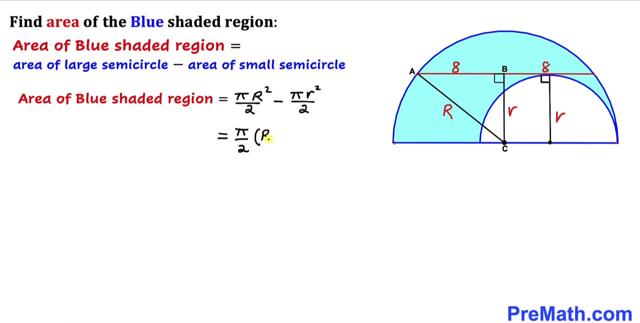 outside. so we are left with R square, the uppercase R squared minus the lowercase R squared. we call this our equation number one. and now let's focus on this triangle ABC. and we know that this is a right triangle. so therefore, we are going to use the Pythagorean theorem. and here's our Pythagorean theorem: a square plus b. 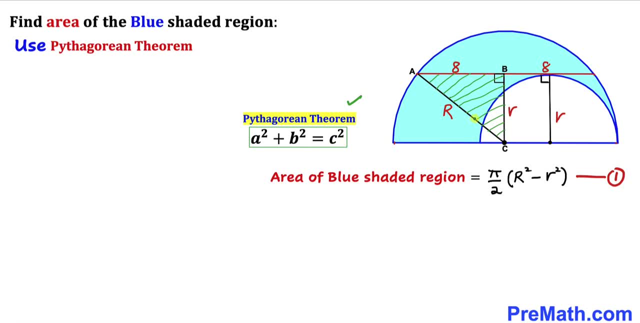 square equal to c square in our case. this is our longest leg. let me go ahead and call this side c. I'm going to call this side lowercase a and this our lowercase b. now let's go ahead and fill in the blanks in this Pythagorean formula: a, in our case, is 8 square plus b, in our case, is lowercase. 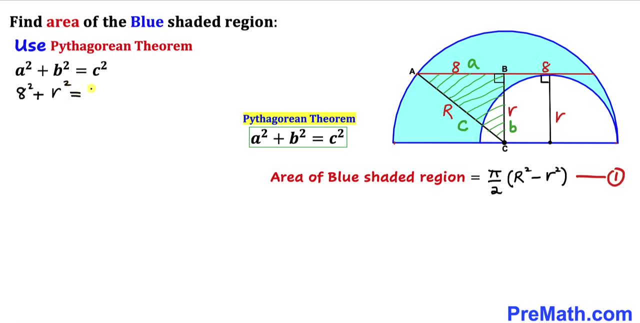 r, so it's going to be r square equal to uppercase r square. let's move this r square on the right hand side, so therefore, we are ended up with the uppercase r square minus lowercase r square equal to 16.. Now let's focus on this equation one. we have r square minus r square. I'm going to replace: